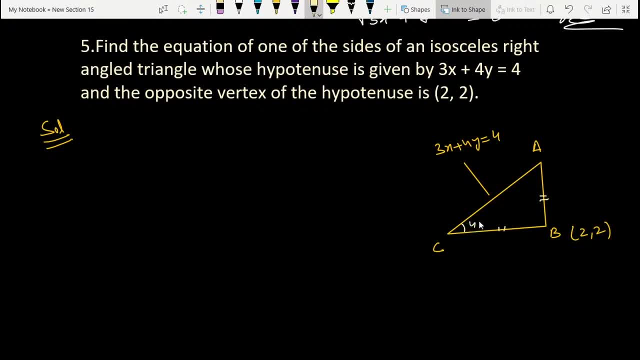 So its every angle will be 45 degree, Because triangle is an isosceles triangle. An isosceles triangle is an isosceles right triangle. Therefore, angle A and angle C will be 45 degree. Now what we will do is Let The slope of BC 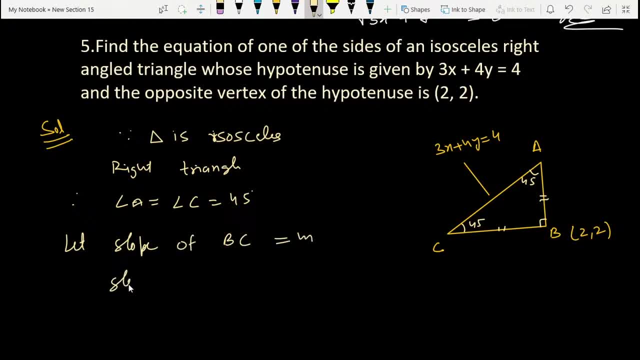 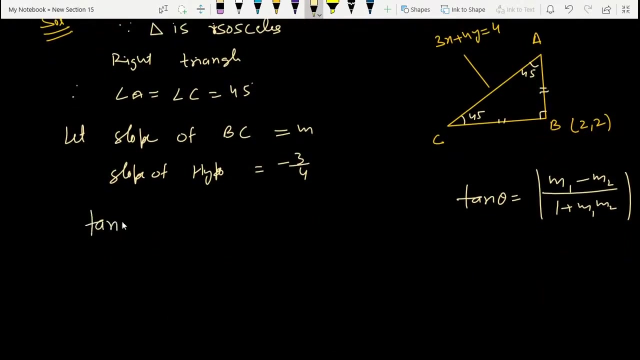 Let's assume the slope of BC is m. After this slope of hypotenuse, We are given Minus 3 by 4 Angle between two lines. We will apply its formula, We will take out m and then the equation of BC will come. M is equal to m by 2. 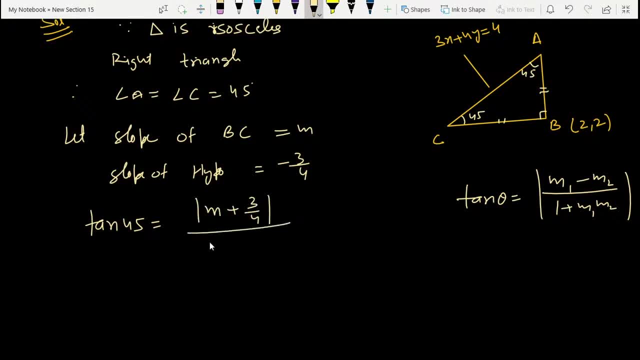 The slope of BC is m by 2. The slope of BC is m by 2, So it is 1045. M is equal to m by 2, And then it is 1045. So 1045 is equal to mode of m. here minus will come 1045, 1. so here plus minus 1, 4m plus 3 upon 4 minus 3m. so let's take 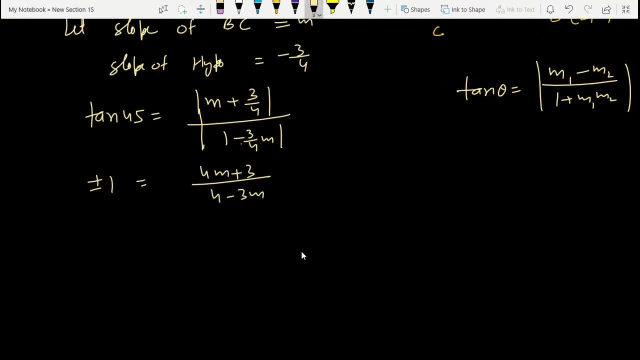 the value of m. so 4 minus 3m equal to 4m plus 3, and minus 4 plus 3m equal to 4m minus 3. so here the value of m came 1 by 7, and here the value of m came minus 7. now we have m. 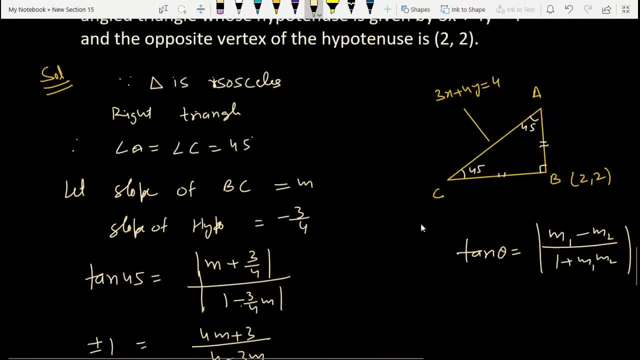 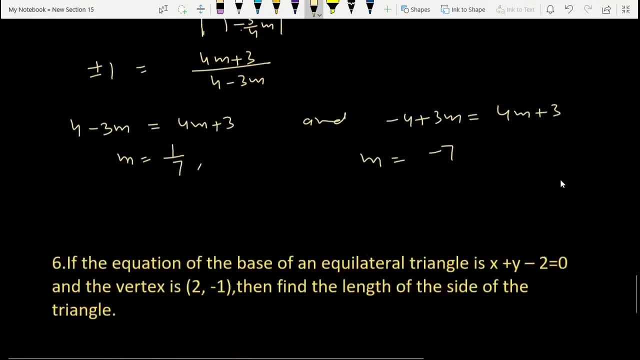 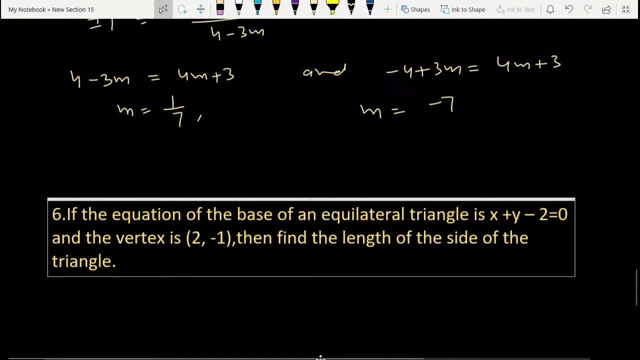 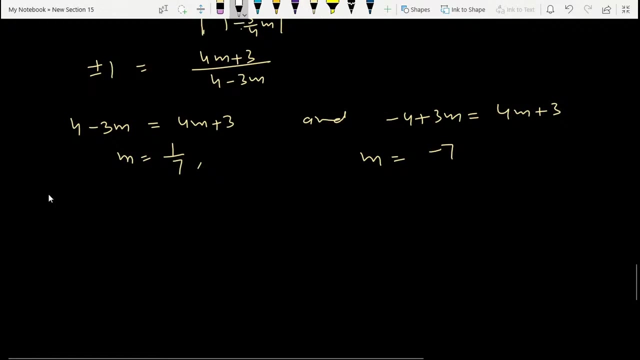 slope, means if we take the slope of bc 1 upon 7, then it is clear that ab will be 2o minus 7. this is its opposite. so if we take the equation, if we take m, then what is the equation of ab? equation of bc? 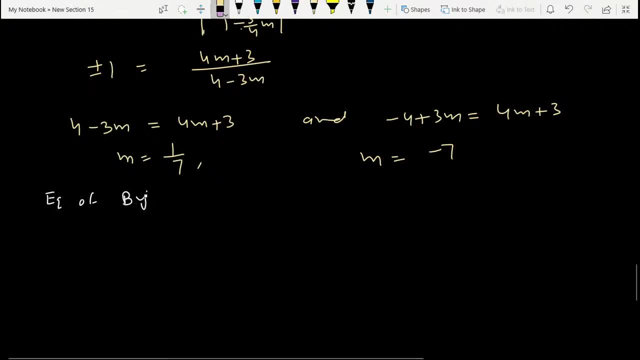 equation of bc is y minus y m, equal to m x minus x 1.. because m is in the point now, the answer is right. because m is in the point now, the equation of bc is equal to equation of x: 1 plus m x. 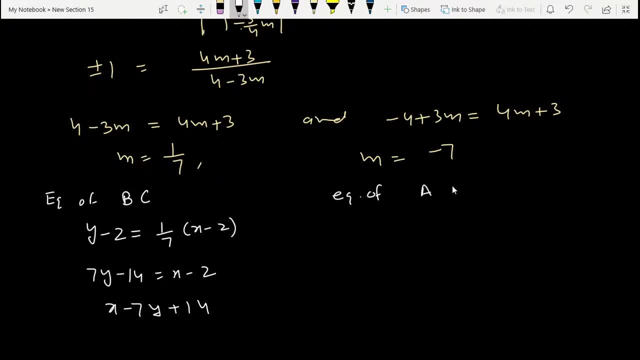 minus x, 1.. a, c, a, b. sorry, equation of a, b will be slope minus 7, so y minus 2 equal to minus 7 or x minus 2. so we will take b- previous equation- as y equal to b. our answer is last or whatever. 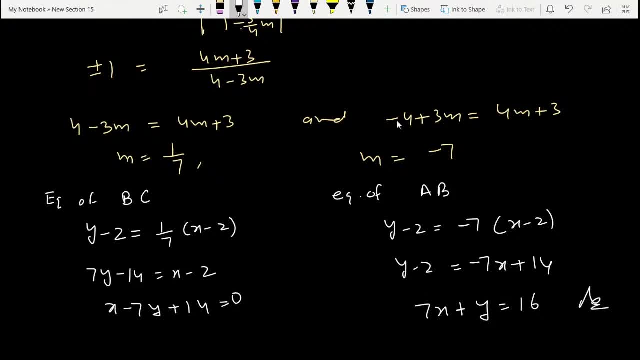 you see, we call it as superscript, so if my using lines doesn't match, then we can write: key of b asARTy Chinese four powers minus three, equal to. with the help of formula we Ο 12, and other functions also are shown. So you get: 1. See w or cotts in nichtаемwhy to 6a. here it makes some picture like if we oppression of W in SubHistory, yyou, shallness and schismyou shall not get any expression of理. Thank you, RubyI hope u try to draw it. correctlyso w and obviously followed the letter e-book. What's the most?